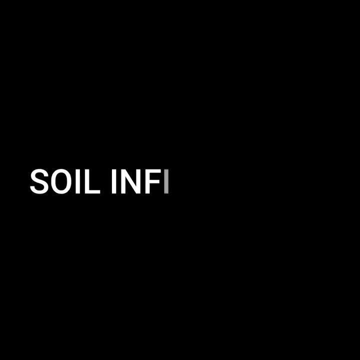 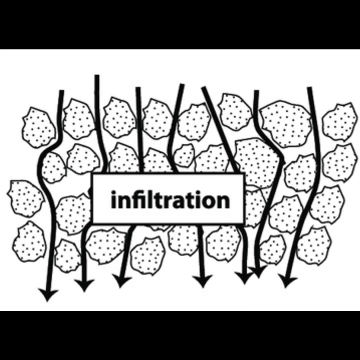 Hello, In this video we will be learning about soil infiltration and why it is important to soil health. What is soil infiltration? Well, it is the movement of water into and through the soil. It allows the soil to temporarily store water, making it available for uptake. 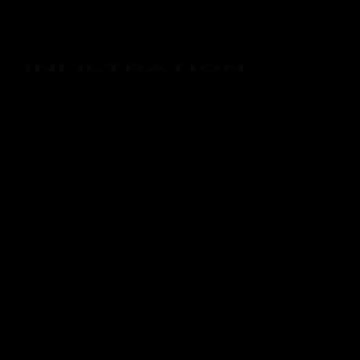 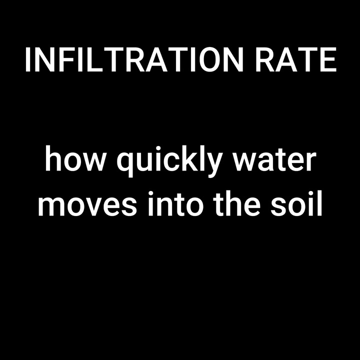 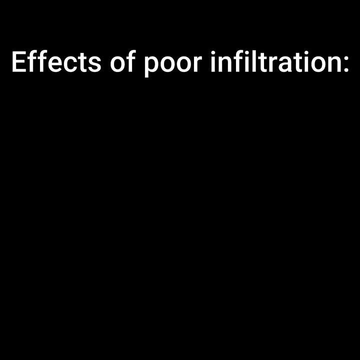 by plants and soil organisms. What is an infiltration rate? The infiltration rate is how quickly water moves into the soil. There are many effects that poor infiltration rates can have. Slow or no infiltration can lead to ponding, which can harbor bacteria and house mosquito larva. 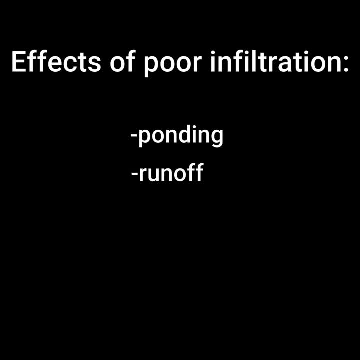 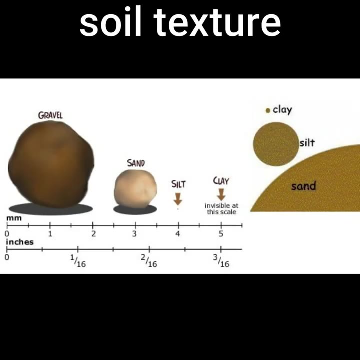 or it can cause surface runoff, which can lead to erosion and loss of nutrients. An infiltration rate that is too high can lead to leaching. So what affects soil infiltration? Well, soil texture is the number one thing that affects infiltration. To review. 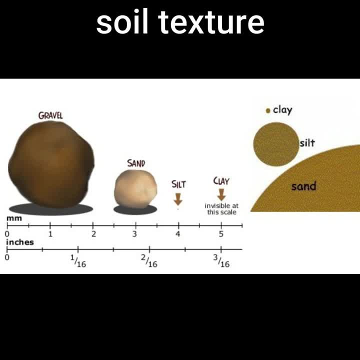 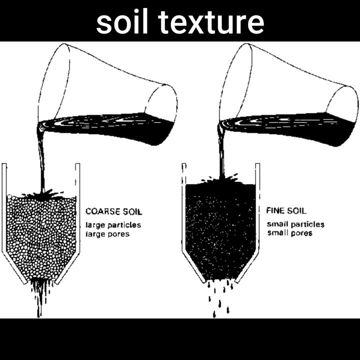 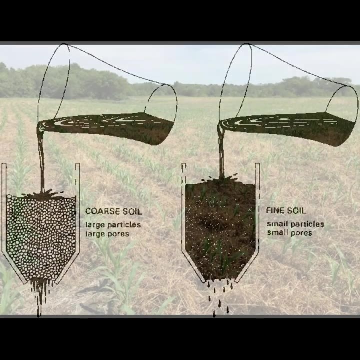 soil texture is the proportions of relative particle sizes. So water moves more quickly through large pores of sandy soil than it does through the small pores of clay soils, especially if the clay is compacted and has a large amount of moisture. The soil texture of the soil, which is a very massive volume of water that is often 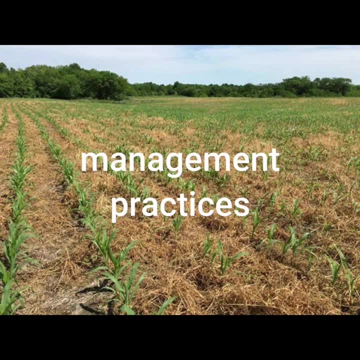 cut down would collapse. For example, water flows quickly back to a solid soil and may break the composting process. The layer of water will oftená tend to show and expectedrá affect soil structure in fashion by lot more from soil size instead of from you know. star thickness or só 국민 dilナ poots pessoalá. dimension. The soil texture. can��аз the soilытó responsibilityは the ideal temperature to do anything for land use? Manageant practices also impact soil infiltration. Management practices such as providing ground cover and managing equipment. traffic impact infiltration by affecting surface crusting, compaction and soil organic matter. Soil most often affect soil drama or mean with soil age problems. 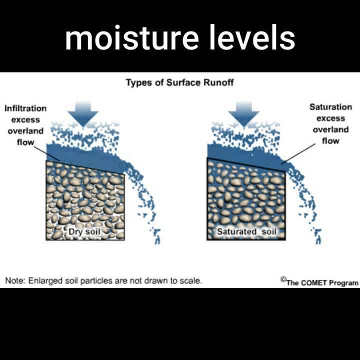 feedback generation may cause soil muftigallo sim melody loss muogether soil moisture saintlôi levels also have relationship with SUNkeit demanded in surface surfaceเร Dylan B scratch and cracks that allow water to enter faster than wet soils As soil moisture levels increase. 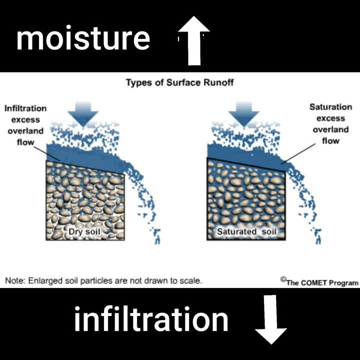 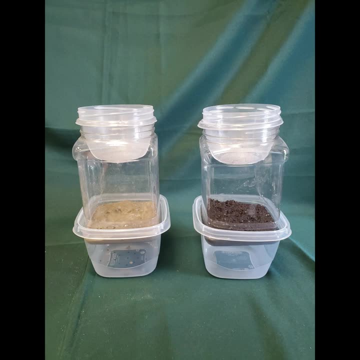 infiltration rates decrease. Soil moisture is impacted by water uptake by plants, residue and vegetation cover, irrigation practices or drainage. I have an infiltration rate demonstration of healthy and not so healthy soil. You can set this up at home if you would like. 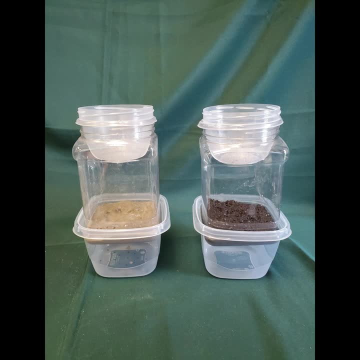 You will need two small containers that nestle inside a large container, which then nestles inside a smaller container on the bottom, like this setup that I have here. The top two containers need to have small drainage holes, similar to a watering can. You will need to place soil samples in the 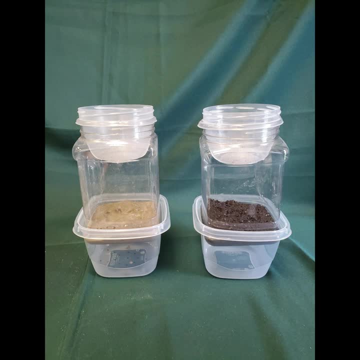 middle two containers. It is best to get two samples, one healthy and one unhealthy, but make sure they are the same texture so you can compare the two. And then you will also need two containers with water in them To do this demonstration. 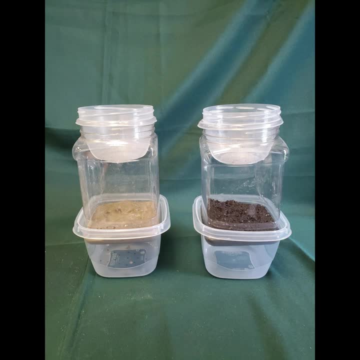 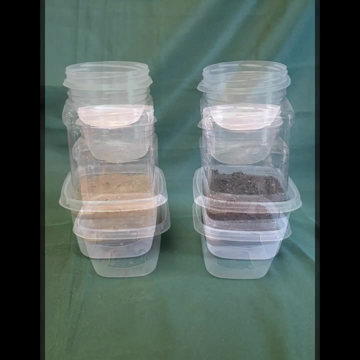 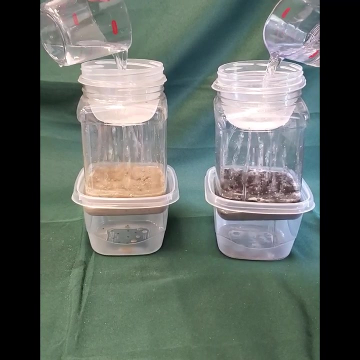 it is best if the soils are saturated and there are no cracks in the soil. Pour water over the samples to saturate them and discard any water that drained through To do the demonstration pour one cup of water into the top. at the same time, Observe what happens during the rainfall. 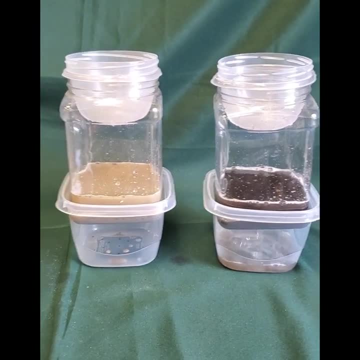 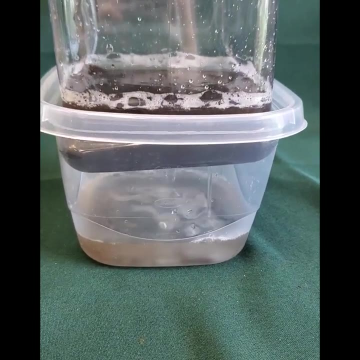 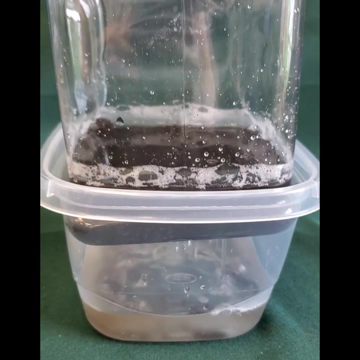 simulation: As the water comes down, the soil sample on the right absorbs the water, and then the water is infiltrated into the bottom container. Looking at the water, you can see that it is fairly clear. Now the container on the left is a little bit different story. The water is not infiltrating. 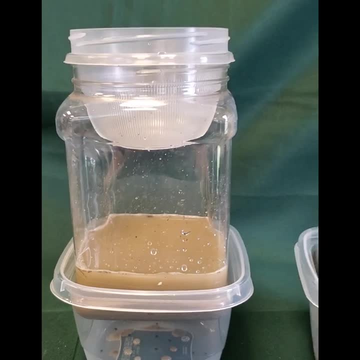 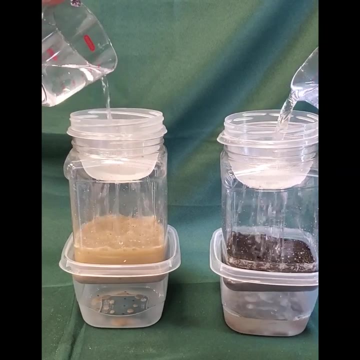 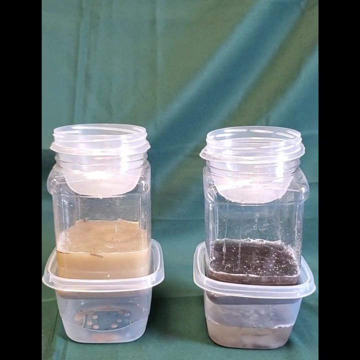 into the soil sample and there are a few drops that have come through, but they are really dirty. Even as we pour more water on the samples, they do the same things. One comes through and is clear, and the other one doesn't come through and when it does, it is really cloudy. Based on this demonstration, the sample on 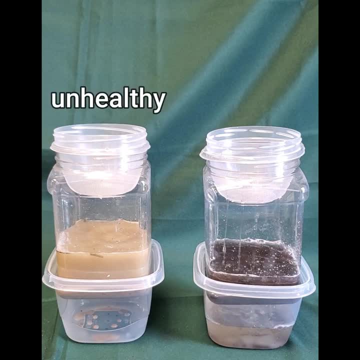 the left would be considered unhealthy and the sample on the right would be considered healthy. Thanks for watching.